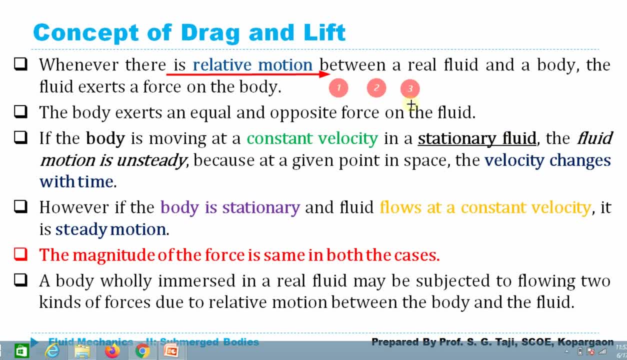 moving with a certain velocities. So if I consider a second case, where my body is moving with a constant velocity and fluid is stationary, this case will be treated as a unsteady motion condition because we know that at a given point in space my velocity is going to change with respect to time. But 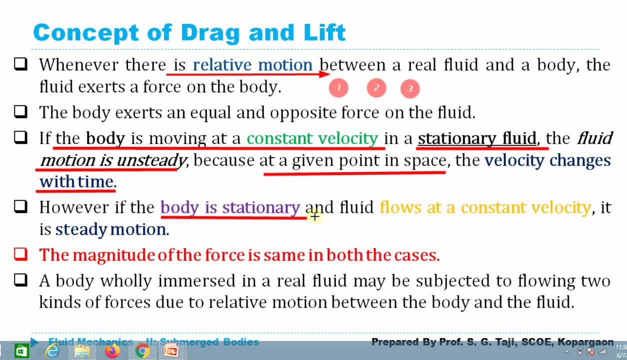 at the same time, if I am considering the first case where my body is stationary and fluid is moving with a constant velocity, this condition or this case will be treated as steady motion. But remember, as we have discussed previously also the magnitude of force is going to remain. 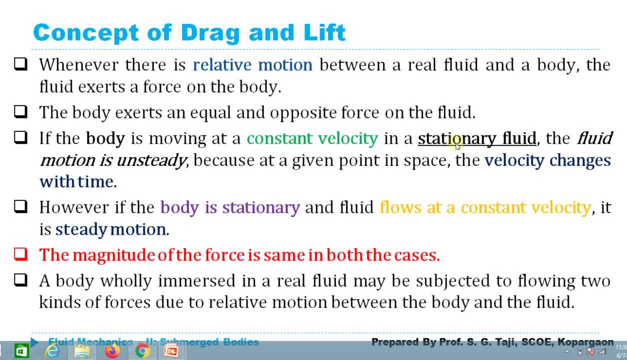 same in both the cases. Now, whenever my fluid is exerting certain amount of force on the liquid, at the same time my body is also going to exert equal and opposite force on the fluid, according to Newton's second law of motion. and this force will be there only because 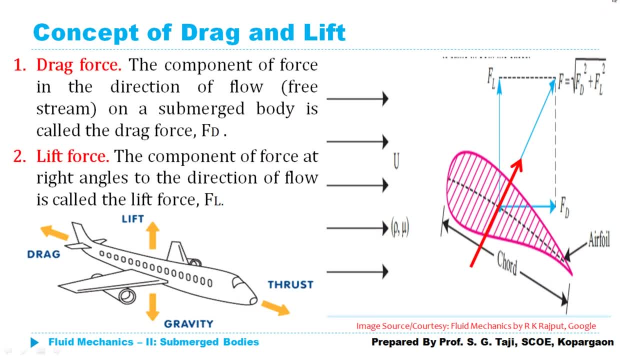 of relative motion of the object and flowing fluid. And now let us consider one body having an aerofoil shape. This body is tropics around it. Imagine that you are moving with an aerofoil on the liquid to which we have immersed in. 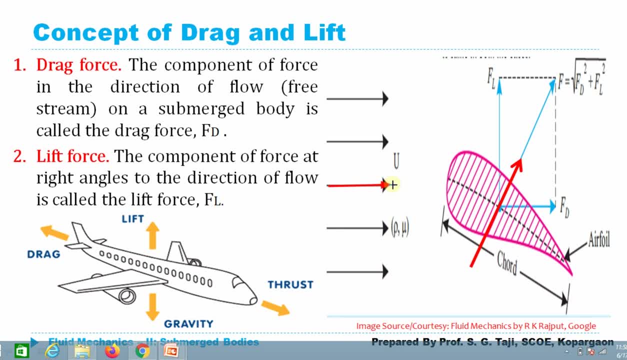 the flowing fluid, which is flowing with the uniform velocity U, having density rho and the viscosity mu, As I am considering here. viscosity, that means that I am considering the real fluid, So I have immersed or submerged this body in the real fluid and whenever this 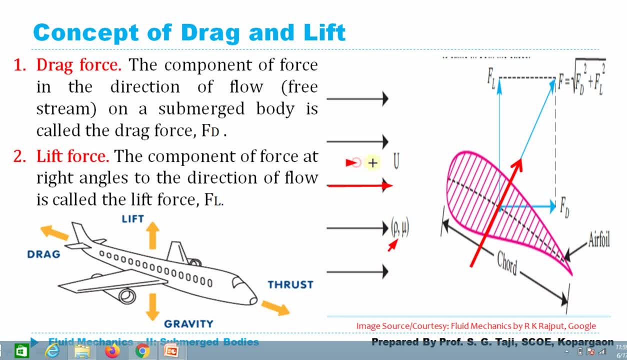 body will be submerged in the flowing fluid which is moving with the velocity U. at that time, certain amount of forces will be exerted by that moving or flowing liquid or flowing fluid on this particular object. In this particular object, there is a point at the moment which is moving around And 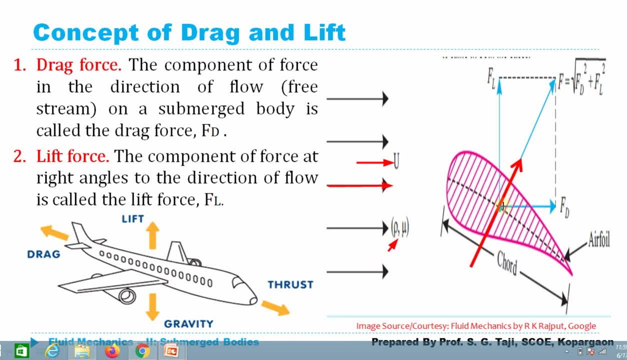 then the mass moving, which is going to be the mass of the liquid, that is, the called. and if I resolve this particular total force in two direction, one component will be in direction of motion or in direction of fluid flow and another component normal to the direction of motion. I will get like this: now let's 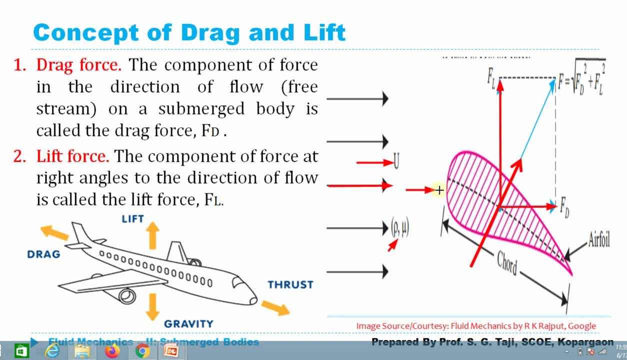 talk about those two components. the first component, that is, a component which is acting in direction of motion, is going to take this body in this particular direction, that is, in direction of motion, trying to push this body in this direction, trying to drag this body in this direction, and that's. 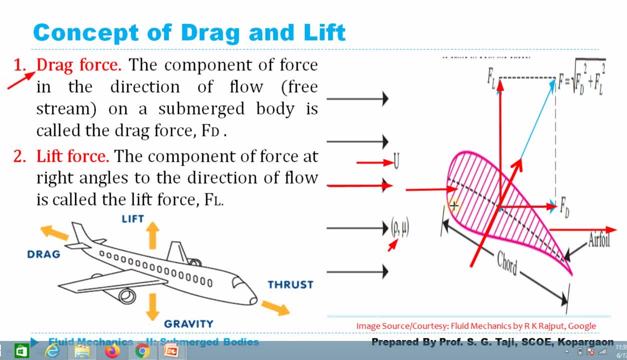 why this force is known as drag force. so this horizontal component of force try to drag this body along with it in the direction of motion, along the direction of motion. now, if I look at the, this vertical component, now this vertical component acting in this particular vertical direction, that is, acting in 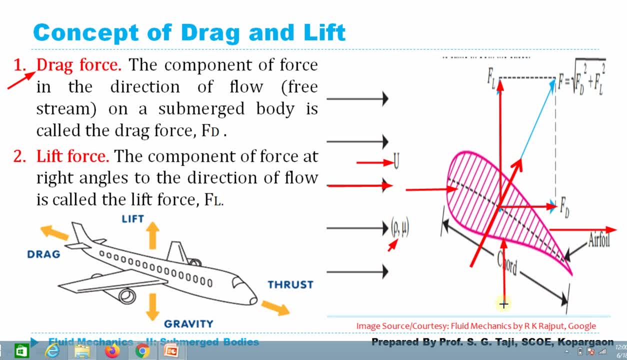 normal, to the direction of motion. what it is doing? it is trying to lift, trying to push this body in upward direction, trying to lift that body in upward direction, and that's why this particular component of the total force is known as lift force. So remember that drag force is the component of total force which is acting along 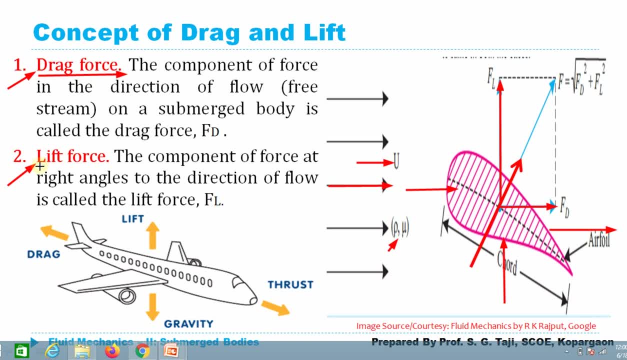 the direction of motion or in the direction of motion, and lift force is the component of total force which is acting normal to the direction of motion, and this is how your aeroplane are generally going to work. Whenever we look at the aeroplane at the time, it will be subjected to. 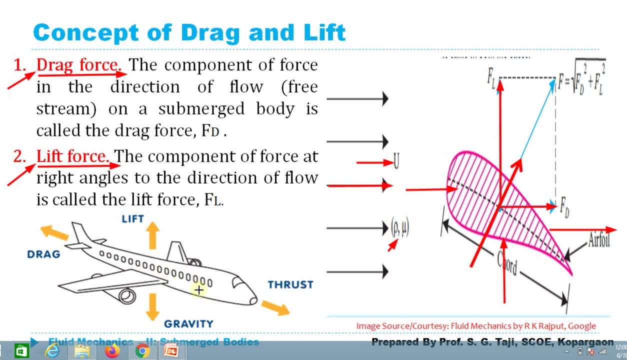 those four forces. Now, whenever this aeroplane try to move in the forward direction, at that time it will be subjected to drag force, which is acting in the backward direction. Now, if we want to keep this aeroplane moving in the forward direction at that time, we need to overcome this. 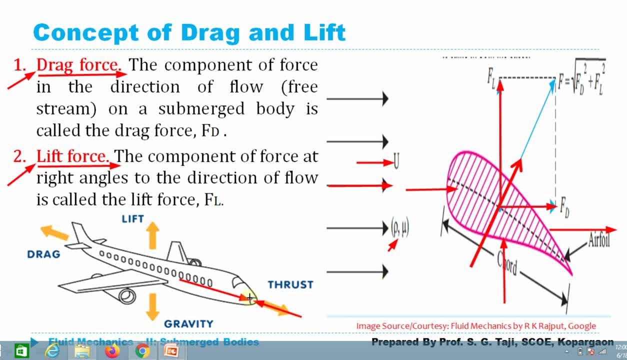 resistance which is provided by the fluid. Now, to overcome that resistance, we use those jet engines where the thrust will be generated and this resistance will be overcome and this aeroplane will move in forward direction. At the same time when vertical buoyancy is applied, the weight will be applied to the aeroplane which is acting in the backward direction. 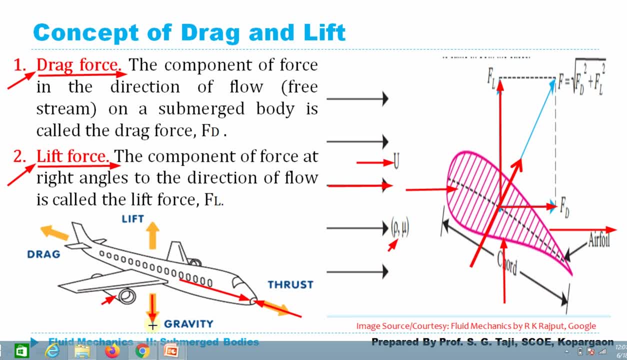 component which is acting downward, that is, weight component of the aeroplane. so to counter this weight component, we use this lift force. by using this lift force and by maintaining this lift force equal to the weight component, our aeroplane able to maintain its flight distance from the aeroplane up to the part at the 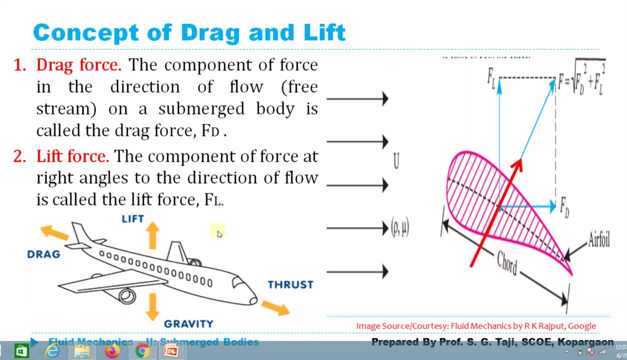 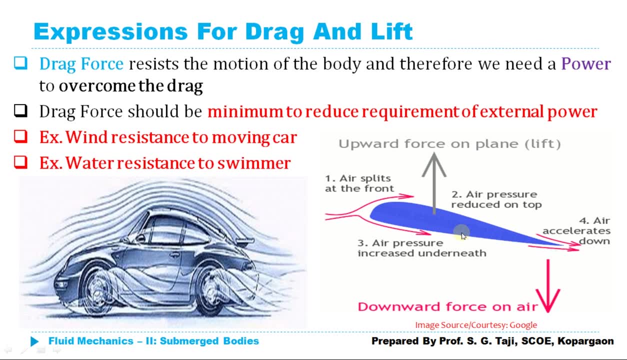 particular altitude. so this is how your aeroplane fly in the sky. again, if we look at the takeoff of the aeroplane, this is how your takeoff will be takes place whenever this particular aeroplane move for in the forward direction and whenever it will take takeoff. at that time it will be slightly inclined to the 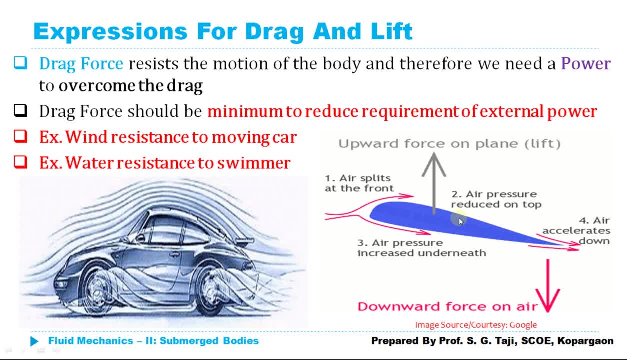 ground and at that time, whatever your air pressure will be decreased on the top side and air pressure will be increased on the bottom side. due to this pressure difference, there will be a generation of lift and your aeroplane will take off in the sky. and same time. if you look at the 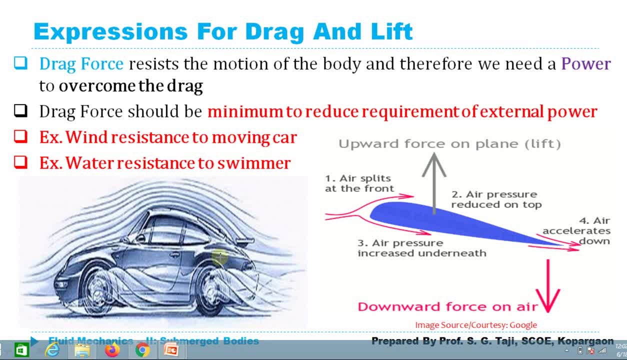 example of vehicle which is moving in the on the road at that time, if you want to keep this vehicle moving on the road and we need to overcome the resistance provided by the air in the backward direction, and that's how, that's what we are going to overcome that resistance by using the power generated by using 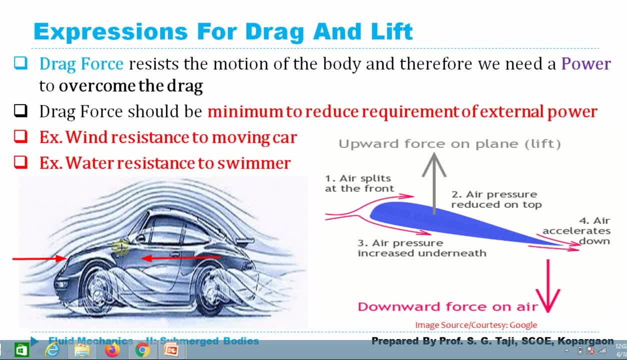 engines and generally we need about 30 to 40% fuel to overcome this air resistance that is provided by, in the forward direction of a drag force, by that particular fluid. so we know that drag force is going to resist our motion of the body and therefore we need the power to overcome the drag and therefore we need to 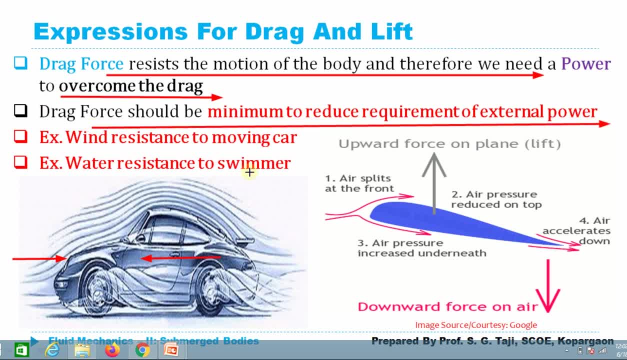 maintain our drag force, to reduce our external power, to improve our efficiency. so we need to reduce this particular drag force. we need to reduce this resistance by proper designing, proper aerodynamic design of the vehicle or of the aeroplane, so our external requirement of external power would be get also reduced. you can also take an example of a water resistance to the swimmer. 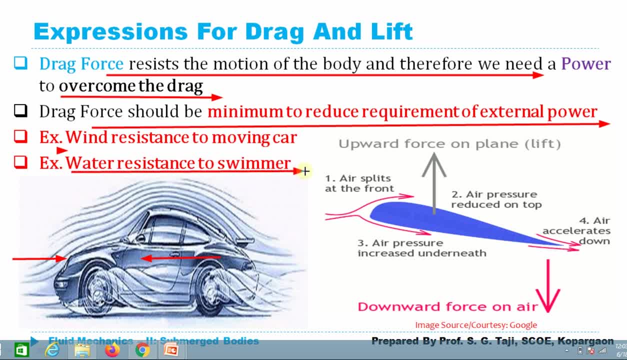 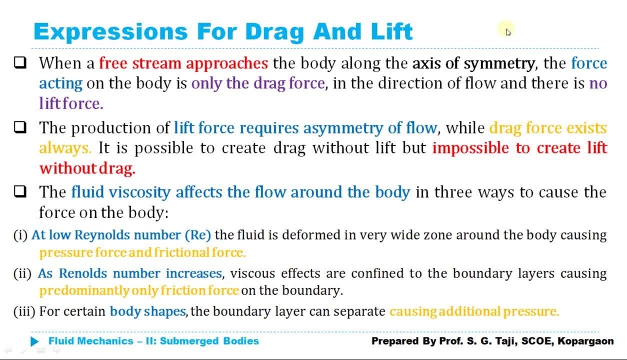 they are also going to face that, going to experience that resistance which is provided by the water when they are moving or swimming through the water. just few things. we need to remember about the drag force when my free stream approaches to the body along the axis of the. 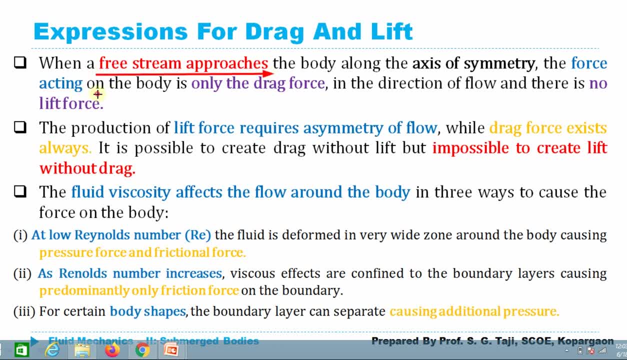 symmetry. at that time time there will be only a drag force which is acting on the body and there will be a no lift force. now, if you see here, we know that whenever my total force which is acting on the particular object, if i am considering any object which is moving through the flowing liquid or flowing, 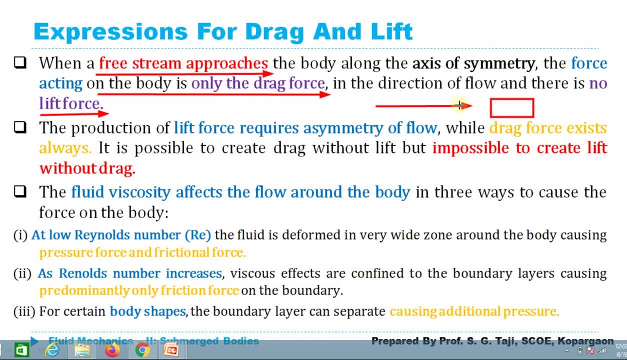 fluid, at that time, if its axis of symmetry is getting coincide with this total force, at that time there will be no lift force. because we know that if your total force acting within certain angle, if our total force is acting within certain angle, then whatever its horizontal component will. 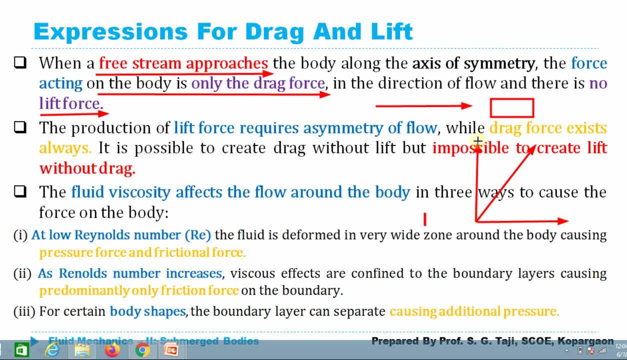 be known as drag force and vertical component will be known at lift force. but what if my, this total force, is acting in horizontal direction? in that case there will be no vertical component. if there is no vertical component, there will be no lift force. again, we know from the discussion. 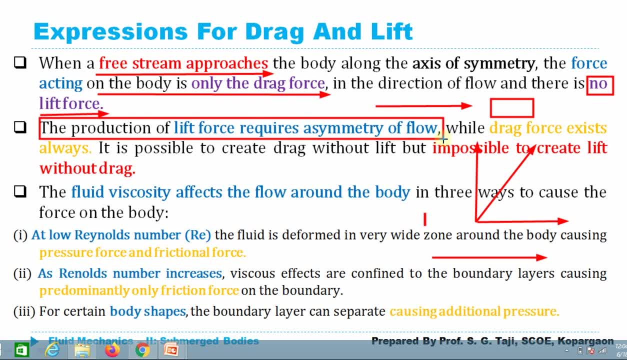 we can say that to generate the lift flow we need a symmetry of the flow. that is, we need to act this particular total force, we need to act this particular total force at a particular angle. then and then only we can produce a lift, otherwise there will be. 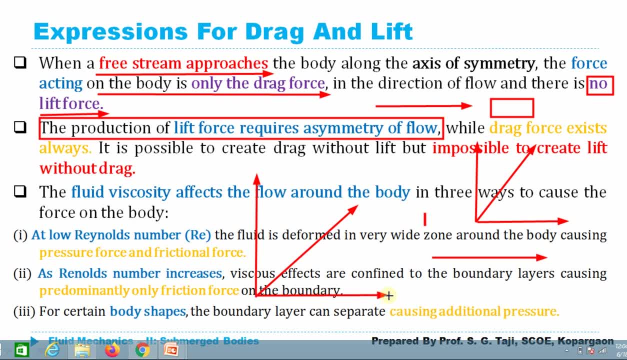 no lift, because there is no, there will be no resolution of the force and if there is no resolution there will be no vertical component. so it may possible to create drag force without a lift, but it cannot be possible to create a lift force without a drag force, because this vertical 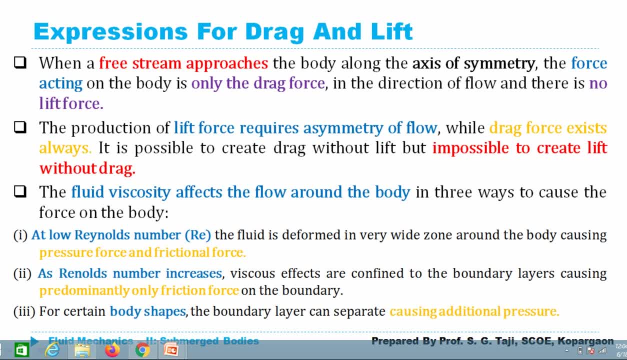 component may or may not be exist, but horizontal component always be exist. if your axis of symmetry is getting coincide with the direction of motion, at that time there will be no lift, for there will be only a drag force. so it is possible to create a lift force without a drag force, because it is. 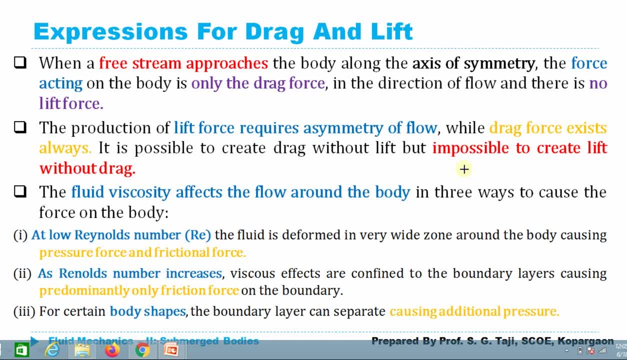 to create a drag force without lift force, but it is impossible to create a lift force without drag force. so remember that drag force always be, exist there, always be there. another most important thing is that fluid viscosity going to affect our flow around the body, as we all know. 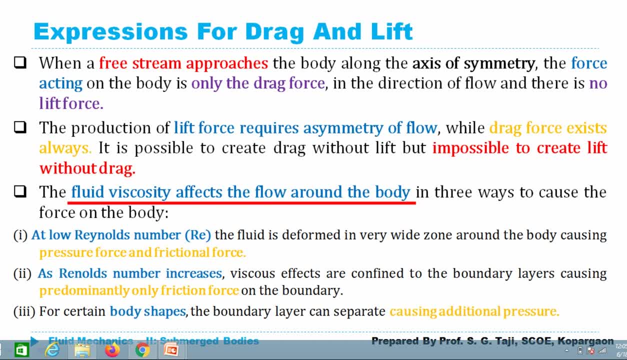 as we have discussed during the discussion of basics regarding boundary layer theory- at that time we also discussed this- fluid viscosity is going to affect the flow around the body. so if you look at the affection that- how it is going to affect, if i look at the low renal number, 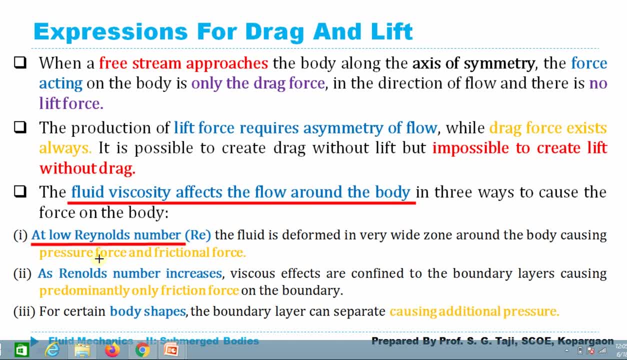 what is going to happen in the low renal number, whatever fluid is going to deform in very deform in very wide region around the boundary, which is may going to increase your pressure force and frictional force. and the low renal number, where viscosity is going to play a major role. whenever my renal number is low, that mean that viscosity will be higher. 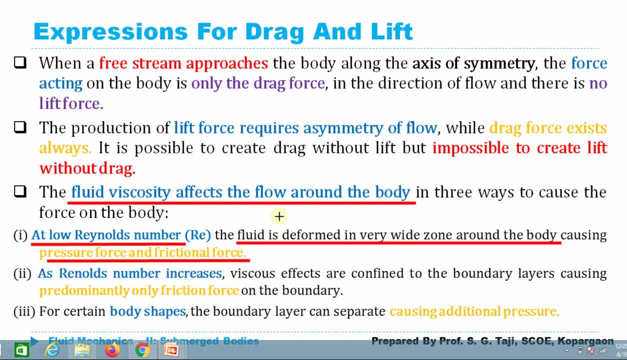 and And in that case, as viscosity is higher, at that time pressure force and frictional force- both are going to play important role or will going to take a dominant role. But if I am considering as my Reynolds number increases, viscous effect are going to decrease.